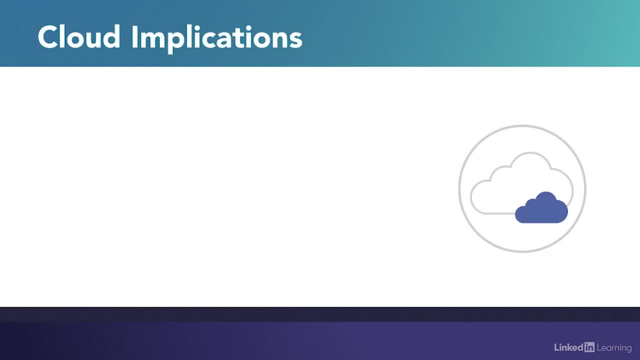 Unfortunately, there are plenty of challenges when conducting incident response on cloud services. The commodity nature of cloud means that it can be difficult or impossible to get support from a cloud service provider in responding to an incident. SLAs typically don't cover incident response support addressing only service fee refund. 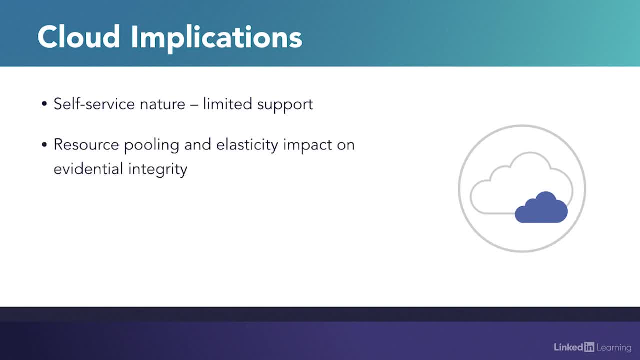 claims. Resource pooling and elasticity may substantially complicate the technical activities of incident response and forensics. Maintaining stability and integrity of evidence when it exists on a shared and still operational infrastructure can be extremely challenging. Results can be extremely challenging. Results can be extremely challenging. 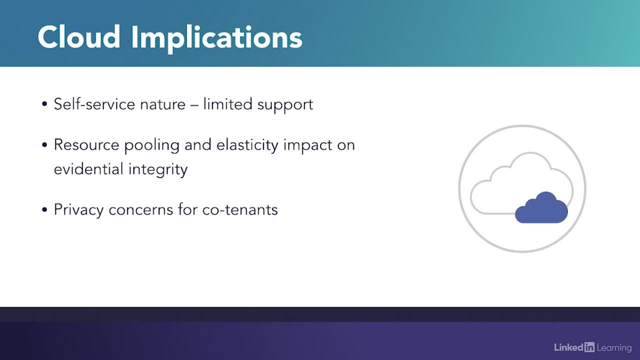 Resource pooling also causes privacy concerns for co-tenants when collecting incident evidence, such as logging net flow data, physical machine images and so on. This can be addressed through filtering out co-tenant information, but that filtering has to be done through a forensically acceptable process. 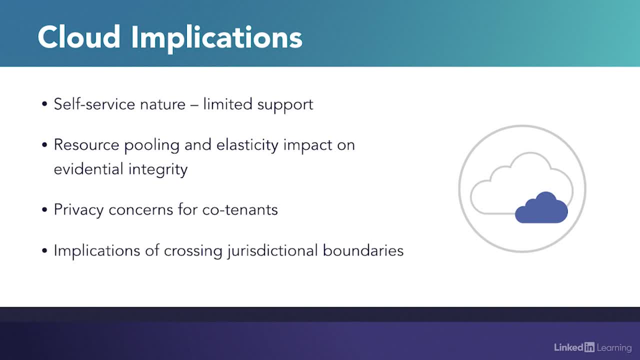 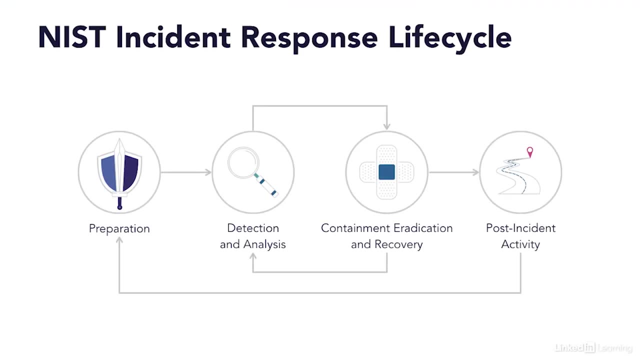 In the cloud data can cross jurisdictional boundaries without the cloud customer being aware. The legal implications of trans-jurisdictional investigations can affect what evidence can be recovered and the extent to which incident response can be effective. The NIST incident response model has four stages – preparation, detection and analysis. 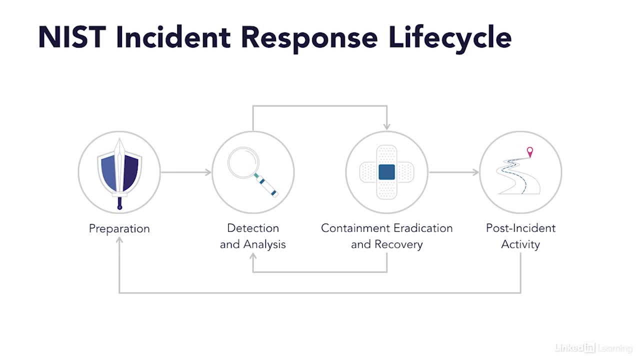 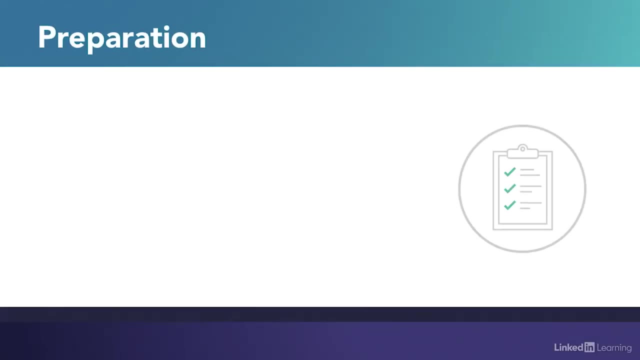 containment, and eradication and recovery. These stages flow from one to another, with some cycling back as the incident progresses and with learnings being used to refine preparation plans. There are four significant considerations in preparation. The first is the key consideration for creating a more consistent experience. 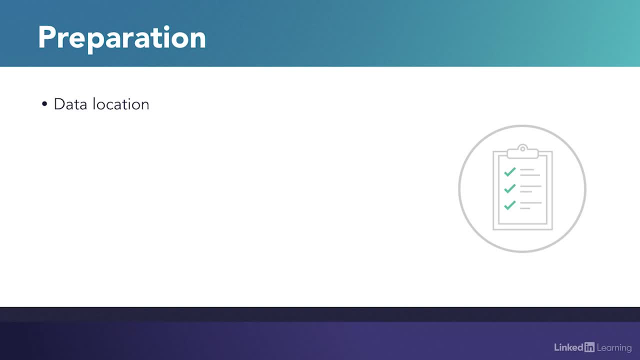 There are three key considerations in preparing for cloud deployment incident response. When designing processes to implement the NIST incident response model, it's important to ensure that the location of cloud data is taken into account. This will have a significant bearing on how investigations and response processes work. 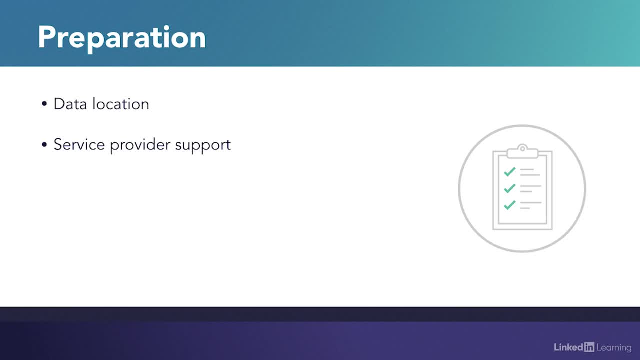 The level of support available from the service provider in the event of an issue will be an important consideration, for incident response is a major cloud issue, then the service provider will be driving their own response, including some level of communication with customers. if it's a customer issue, then the 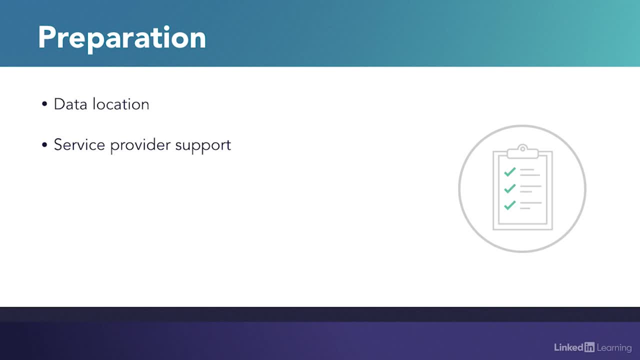 service provider may not be involved at all. threat intelligence is an important source of information prior to any incident due to malicious activity. it can help avoid incidents and can help more quickly identify the cause of incidents that do occur. it's important to establish ongoing access to a data feed of indicators of compromise, the structured threat intelligence and 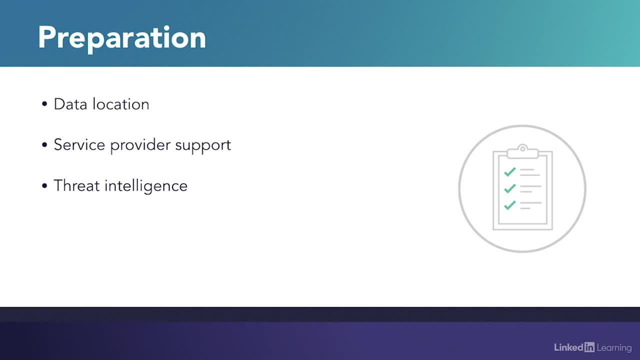 trusted exchange standards. sticks taxi are commonly used for this. the most important part of the preparation stage, however, is testing the incident response process and plan, and the initial exercises can be expected to flush out a number of issues with cloud services. right running cyber incident response exercises will help refine and mature the process. 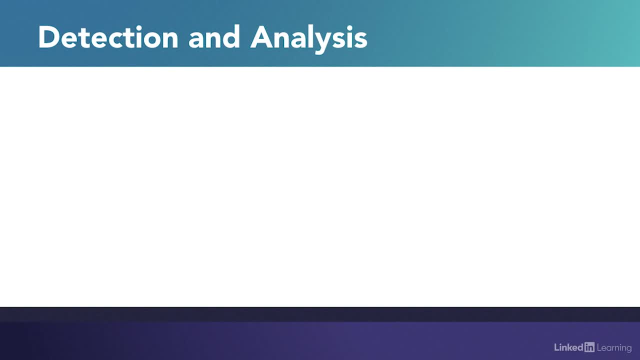 timely detection has a fairly direct relationship to minimizing the impact of an incident. there are a number of issues that need to be considered when designing and operating the incident detection and analysis subsystem. incident detection is based on log data, typically from the enterprise perimeter. in the case of cloud deployments, the source and 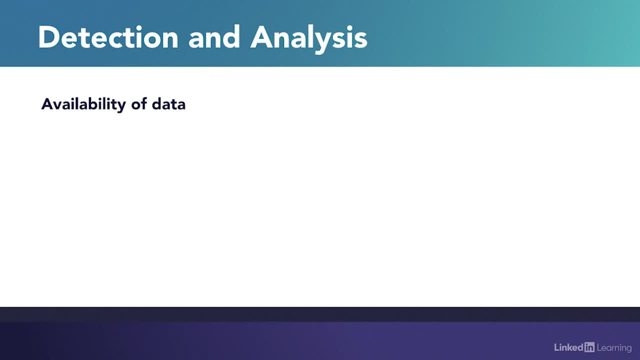 availability of log data needs to be identified. the consistency of data also needs to be managed, particularly around timestamps. both physical and virtual cloud components may change and this can introduce data inconsistencies. it's also important to ensure the correct interpretation of cloud-sourced log data, log retention and availability for analysis. 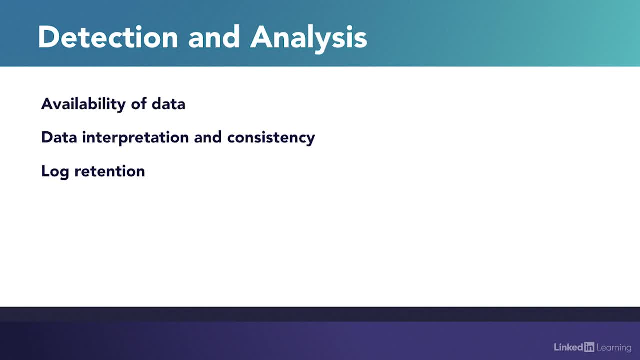 also needs to be considered. given the ability of advanced malware to exist for considerable periods of time before being detected, Forensics will be difficult. Customers will not be able to carry out traditional hands-on forensics on cloud infrastructure and any requirement for forensics. 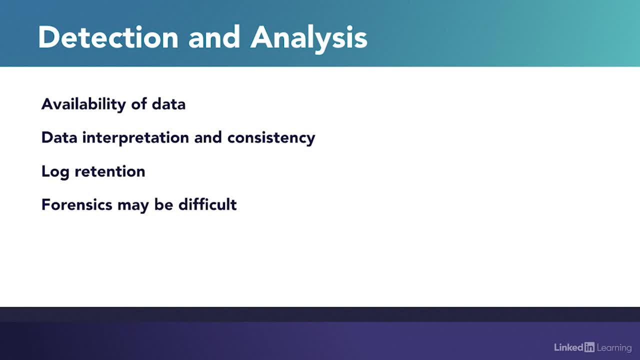 will be limited to the terms and conditions in service agreements. In June 2014,, NIST released the draft NISTR-8006, NIST: Cloud Computing: Forensic Science Challenges. This publication lists 65 problems covering lack of control over and reduced visibility into the infrastructure.